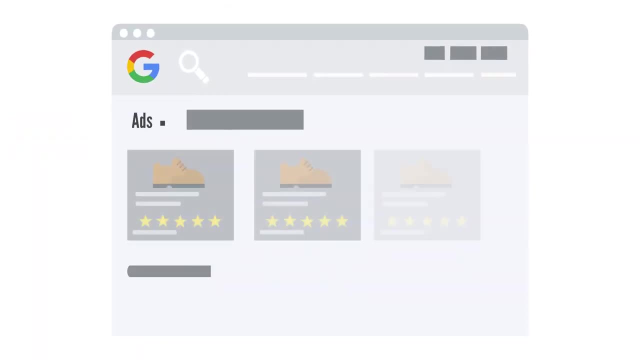 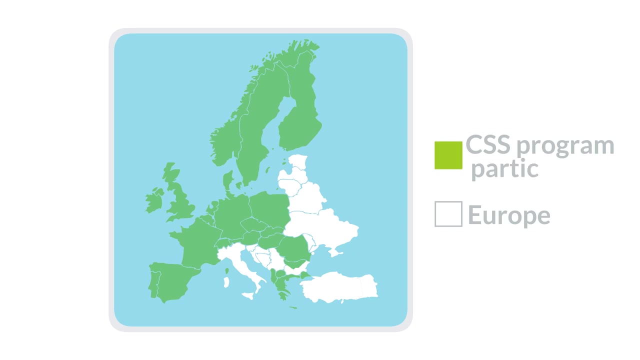 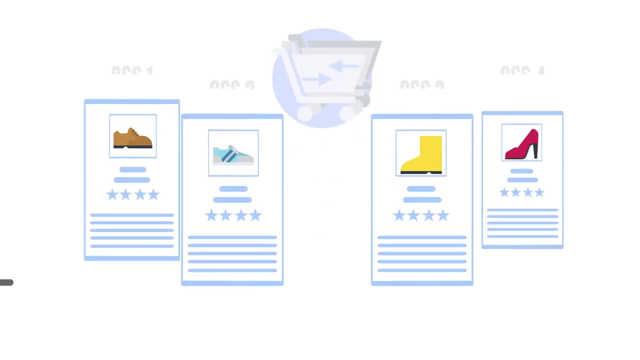 When shoppers search for products on Google, they can see relevant shopping ads for offers from many stores. In countries where the CSS program is available, your store can only participate in shopping ads by using one or several comparison shopping services, also known as CSS. CSS place ads on behalf of merchants and bid for slots in Google's ad auction. 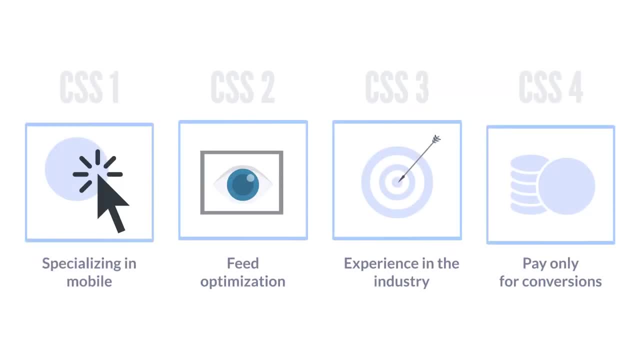 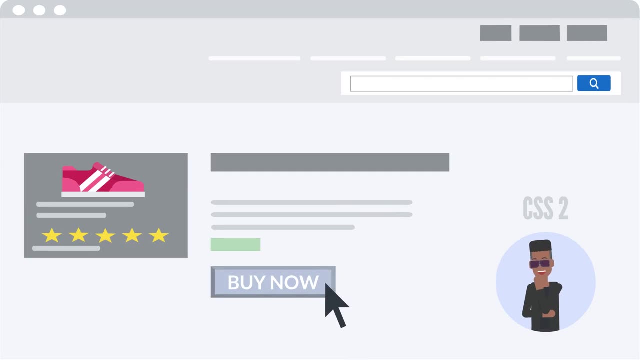 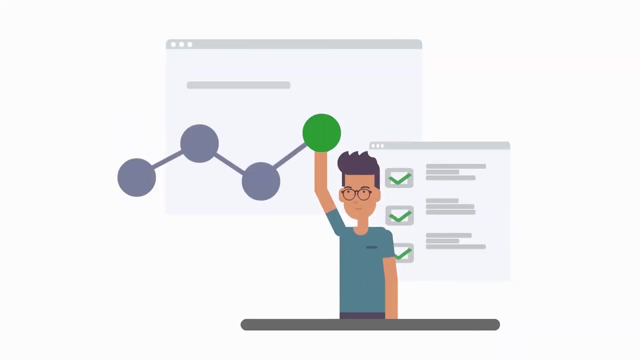 CSS may offer different services and charge for them in different ways. For example, some charge their customers per click, while others charge a commission whenever an ad leads to a sale. Others charge merchants a fixed monthly price as part of the subscription model. Some CSS has managed product feeds and campaigns for you, while others offer a self-service model. 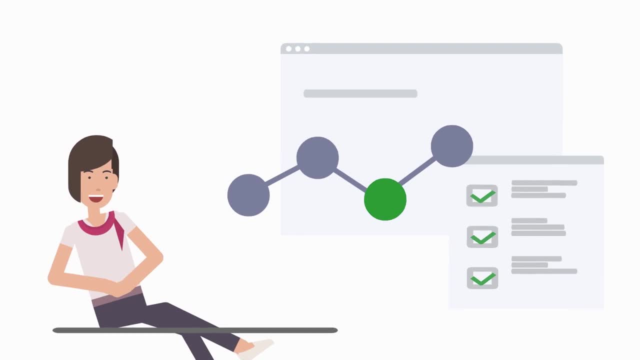 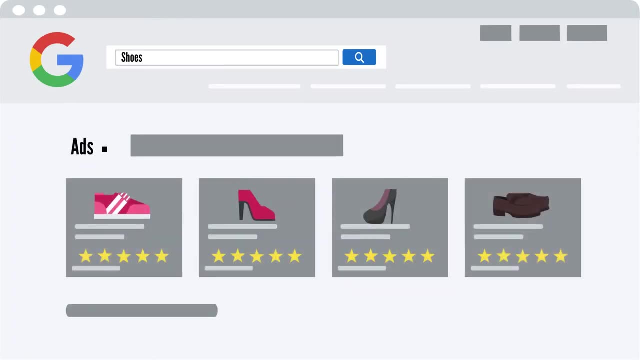 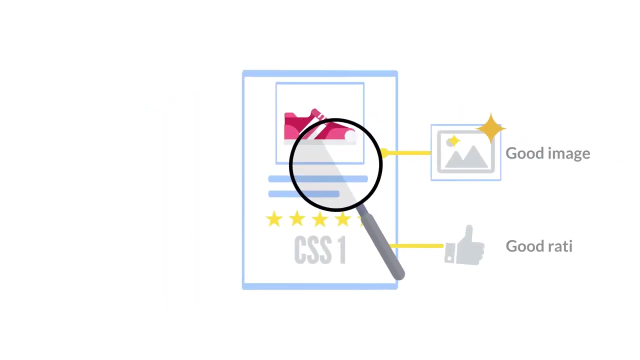 allowing you to address product feeds and shopping campaigns yourself. All comparison shopping services compete equally for ad spaces on Google's general search results pages, and they all have access to the same shopping ad feature. All ads need to follow the same rules designed to make them helpful to users. 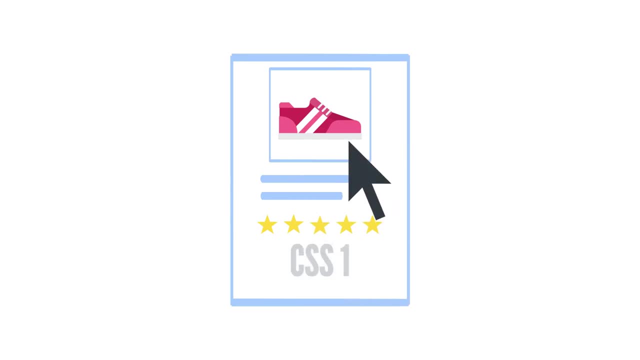 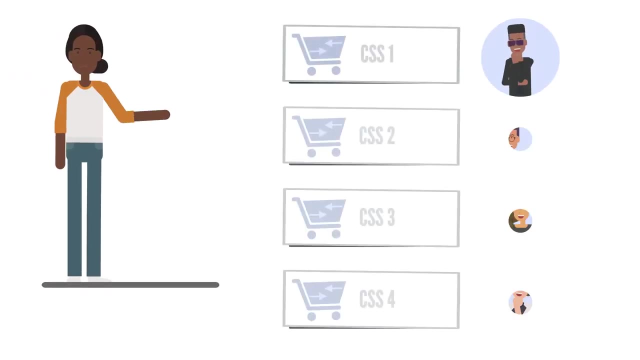 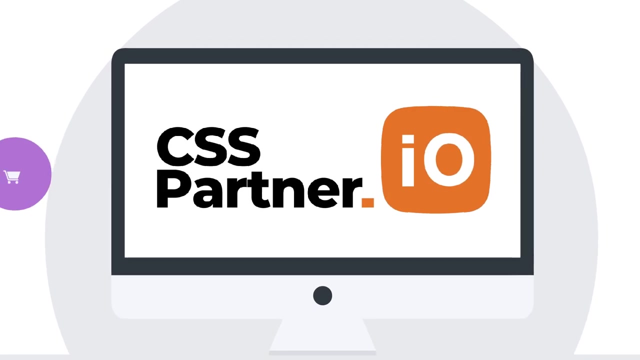 This means, for example, that shopping ads need to take shoppers directly to the store's landing page, where they can buy the advertised product. You can work with one CSS or several CSSes at the same time. CSSpartnerio is your ally to improve the overall performance of your Google shopping ads.